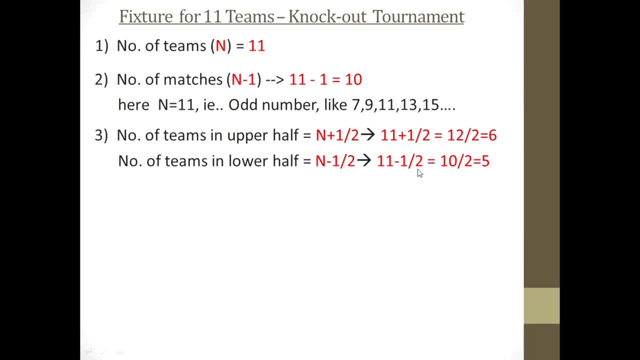 2.. That is 11 minus 1 by 2.. And you will be getting 10 minus 1 by 2.. And you will be getting 10 by 2, that is 5. so upper half there will be 6 teams, lower half, 5 teams. and now coming to number, 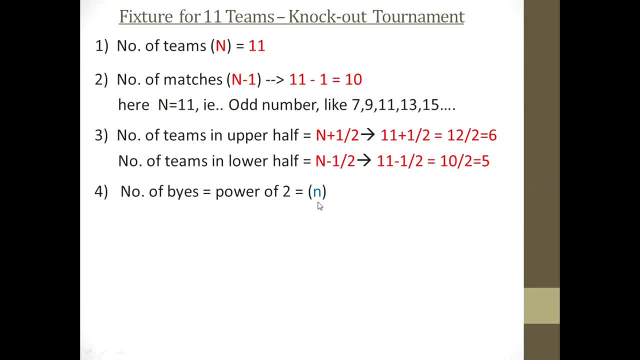 of buys the same. the power of n. we have to see how much we are getting the power of n. that should be greater than 11. so here also we are getting 2 power 4, that is 16. so 16 is greater than 11. 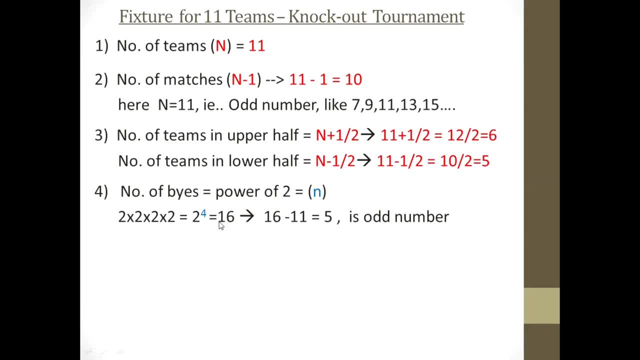 and 2 into 2 into 2 into 2, that is 2 power 4, that is 16. so 16 minus the number of teams you will be getting the number of buys, that is, 16 minus 11, is equal to 5. and here you can see. 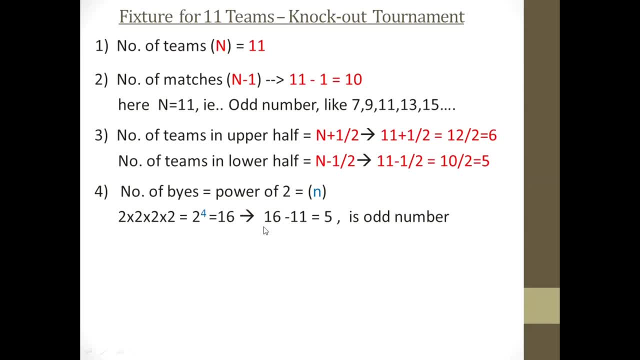 the 5 is the total number of buys and 5 is also an odd number. so total number of buys is represented by b, that is 5, and there are different formula for this. so here you can see that the total number of buys is represented by b. 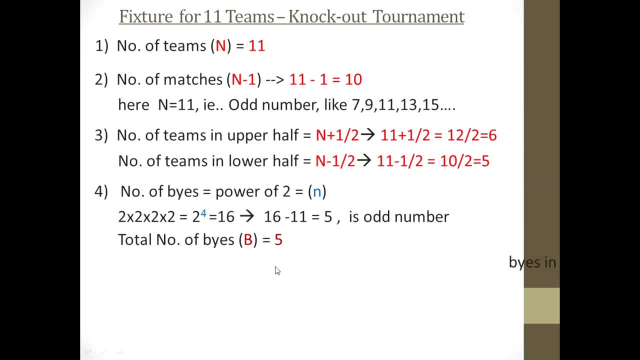 of are the by's also because this is an odd number. so now we have to divide the by's in two halves, so by's in the upper half. here the formula is b minus 1 by 2. okay, that is 5 minus 1 by 2. 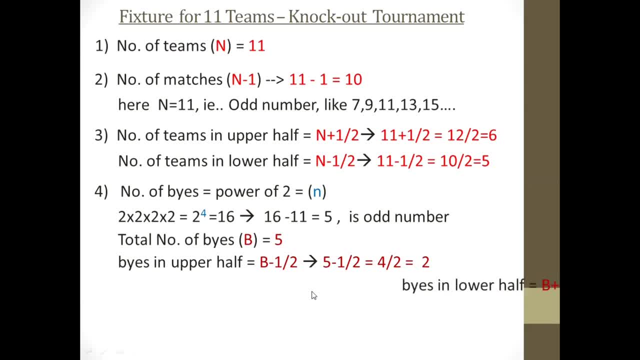 that is 4 by 2, and we are getting 2, 2 by's in the upper half and by's in the lower half. here, b plus 1 by 2, that is 5 plus 1 by 2. 5 plus 1 by 2, you will be getting 6 by 2, that is 3. so 3 by's in the 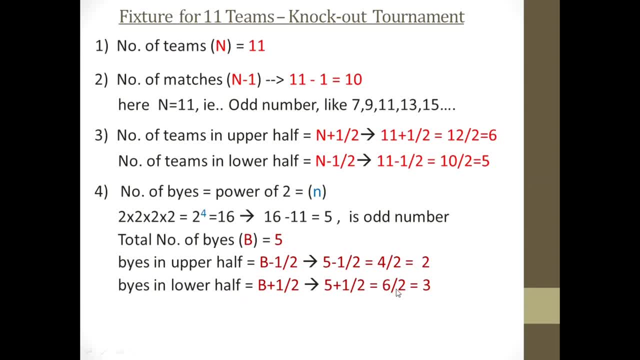 lower half and 2 by's in the upper half. so every time you can see, whenever we are getting an odd number, the total number of by's in the lower half will be more and the total number of by's in the upper half will be less. and now the total number of rounds. so here the same formula for the even. 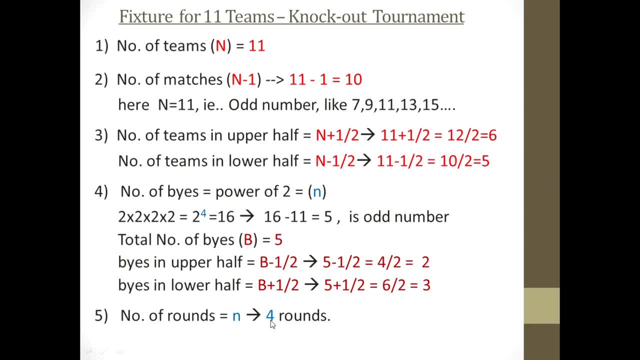 number, also n to the power. So we are getting n to the power 4.. So the n is small, n is equal to 4.. So there are 4 rounds. So total: there will be 4 round matches played in this tournament. 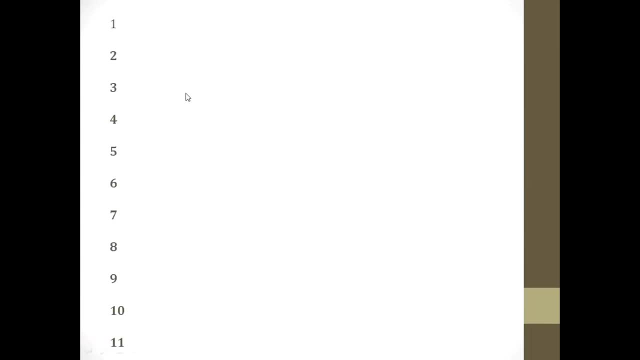 Now how to draw the fixture for 11 teams. Here we are taking 11 teams and the first point is we have to divide into 2 halves. That is, according to the formula, we have got 6 teams in the upper half and 5 teams in the lower half. So we have divided the first. 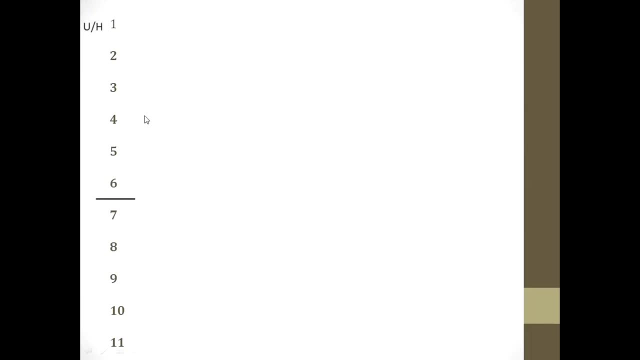 upper half is 6 teams, lower half is 5 teams and this is UH, the upper half, and this is LH, the lower half. So the division of the buys. So first buy is given to the lower half, last team, that is number 11.. The second buy, upper half. 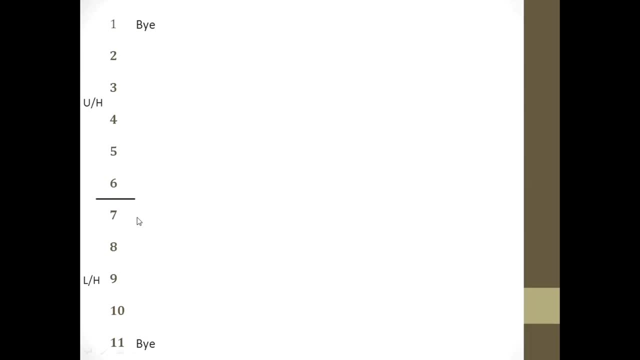 First team and the third buy the lower half- first team and the fourth buy upper half- last team and the next last, fifth buy will be given the lower half, 10th team, that is the last second team. So total there are 5 buys. So 3 buys in the lower half and 2 buys in the 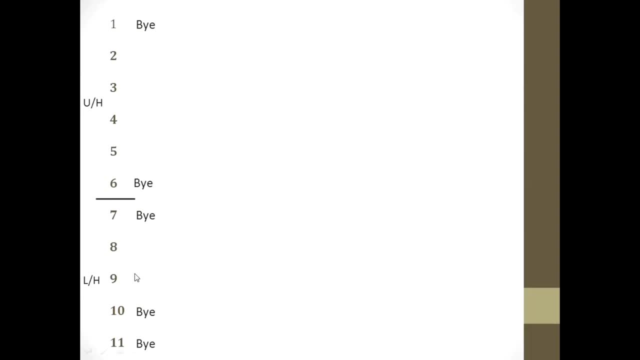 upper half. Now how many teams are there without buys? They will be playing the round 2 and 3. that is match number 1.. We have given with the green color so that it will be easy for you to understand. the round number 1 matches The second match between 4 and 5. that is match. 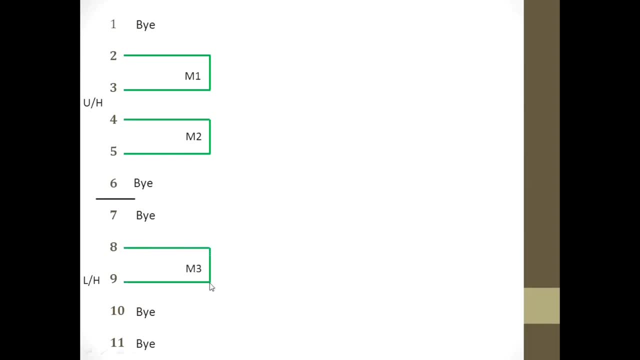 number 2 and the third match between 8 and 9, that is match 3.. These teams are without buys and the buys teams are directly. they will be playing the second round. Now, the fourth match that we have given with yellow color, the number 1.. 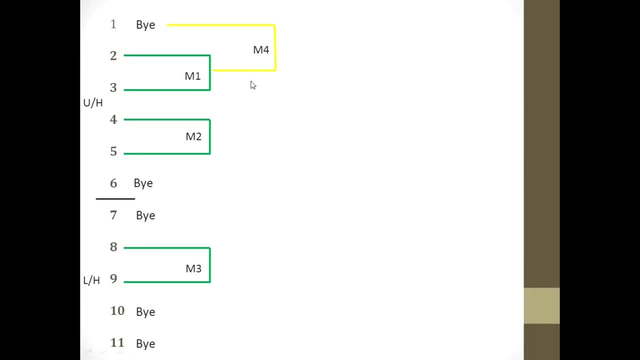 We will be playing with the match number 1 winner, that is, 2 and 3 winner, will be playing with number 1, and the 4 and 5 winner- that is, match number 2 winner- will be playing with number 6, that is, match number 5 and match number 6, the seventh number, that is the buy. 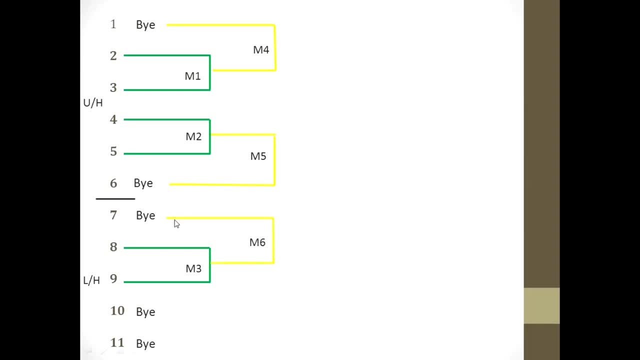 team will be playing with the match winner of match number 3 winner, that is, 8 and 9 winner, and match number 7, both the buys, that is, number 10 and 11.. They will be playing match number 7.. So this is the second round with yellow color And next round 3. It is given with the blue color. So this is match number 4 winner and match number 5 winner.